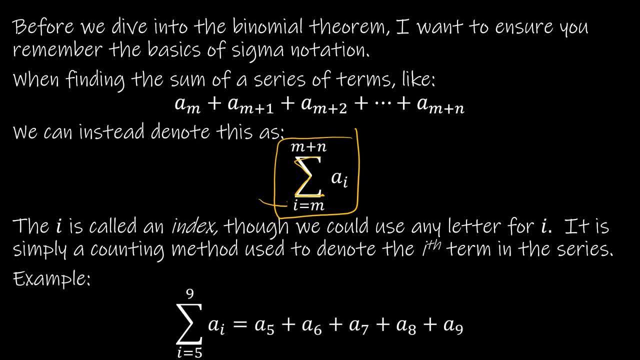 us to find the sum, The value on the bottom and the top. the I stands for index and it's really just a counting procedure. The M tells us the lower limit and the whatever you have up here is going to be the upper limit And the lower limit is going to be the upper limit And the. 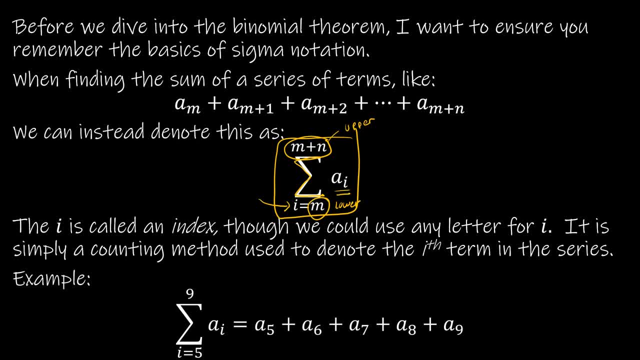 lower limit is going to be the upper limit And the lower limit is going to be the upper limit And the upper limit is going to be the upper limit, And then whatever happens here is really just going to be each value of the series. So if I have this particular series, A sub M, A sub M plus 1,. 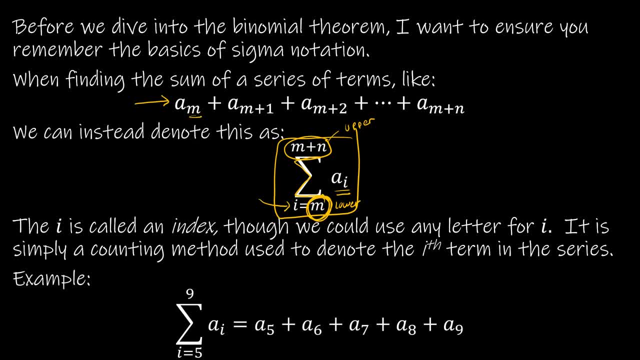 notice that it started at M and then it's increasing by one each time, all the way until we get to whatever our upper limit is. So again, the I is the index and we could use any letter, sometimes K, sometimes J, but a lot of times you're going to see it as I, And then again. 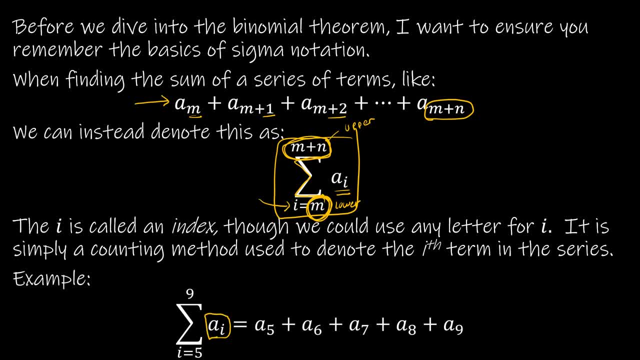 the term here doesn't have to be A sub, anything. It could be, you know, 2 to the 2 times I could be what we're doing, And so then it would be 2 times 5, and then plus 2 times 6, and so forth. 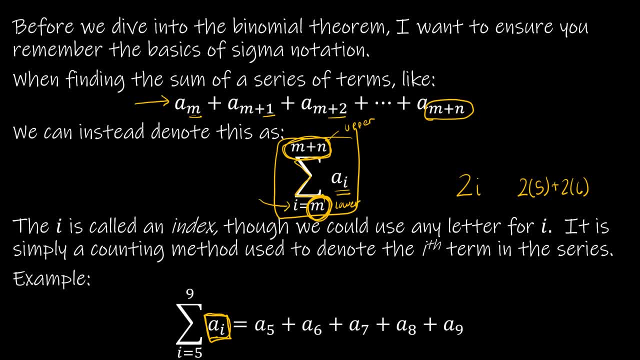 But if it's A sub, anything that's just saying that particular value or place in the sequence. So if I have the summation as I goes from 5 to 9 of A sub, I really it's just saying A sub 5, A sub 6, A sub 7,, A sub 8,. 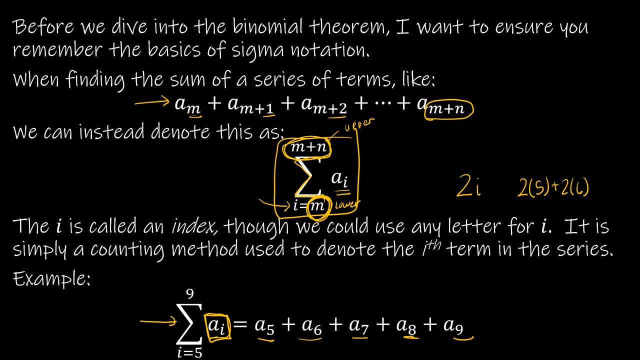 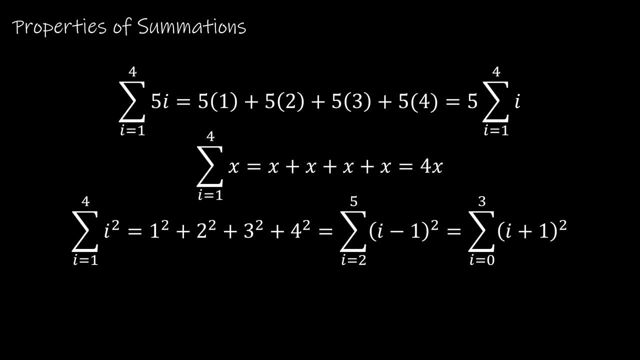 A sub 9.. And you're just going to add those together. We're going to take a look at some properties of summations. We are not going to look at the formulas right now. We will kind of look at those later- But right now I just want to look at a few. 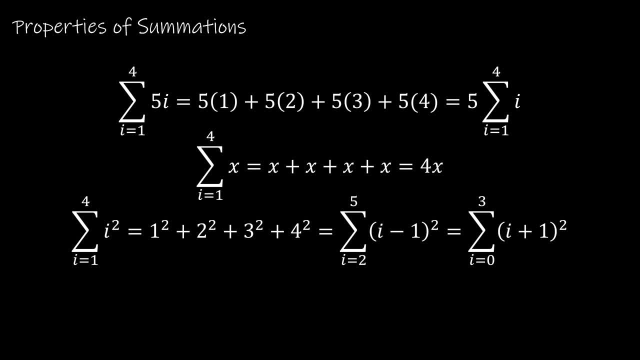 properties that may come into play as we are learning our new material. So the first property is: if I have a summation where I have some constant that's being multiplied by a value, it's the best idea for us to go ahead and take that constant out to the front. So, instead of 5 times, 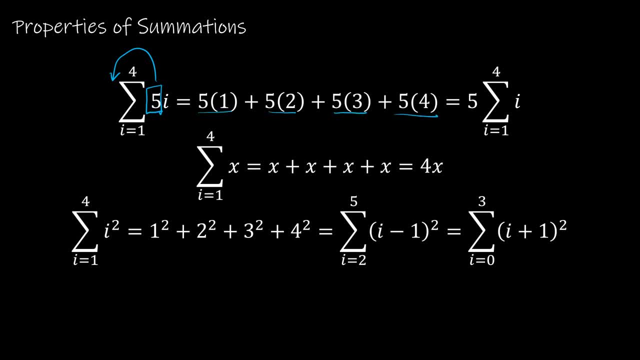 1 plus 5 times 2 plus 5 times 3 plus 5 times 4, again going from 1 to 4, I would just take 1 plus 2 plus 3 plus 4. And then that value would be multiplied by 5. So much easier. The second property is: if you have and 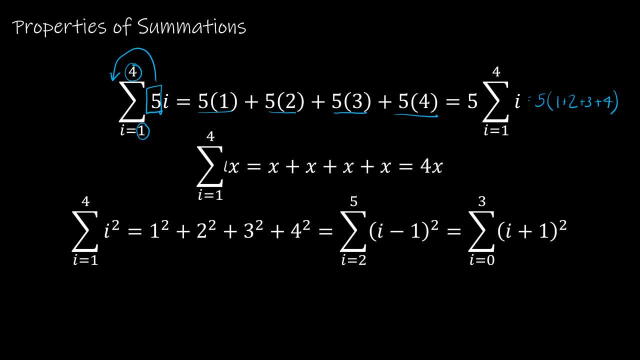 I want you to notice here: in the second expression there is no I inside, So we're not taking the summation of I or anything. So we're just saying we're adding x four times because it's from 1 to 4.. So it's just x plus x plus x plus x. So that property says: hey, if you don't have your index. 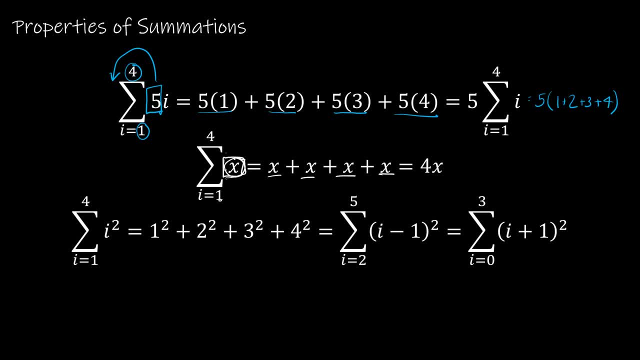 flower in the problem. you can just take whatever you have here multiplied by this value, assuming that you're starting at one. The reason I point out starting at one is right here. You'll find quite often that you have an index and you want to start an index at one, or you want to start it at zero, So you need to be able to know how to. 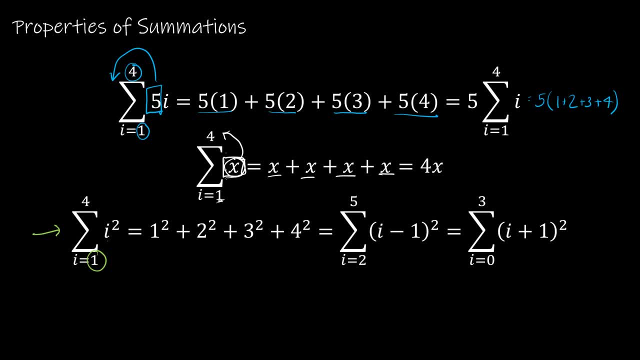 manipulate those. So this tells me: I squared the index from one to four of I squared, So 1 squared, 2 squared, 3 squared, 4 squared. Let's say I wanted my index to start at 2.. Notice, I can add 1 to each of those, so now it goes from 2 to 5.. 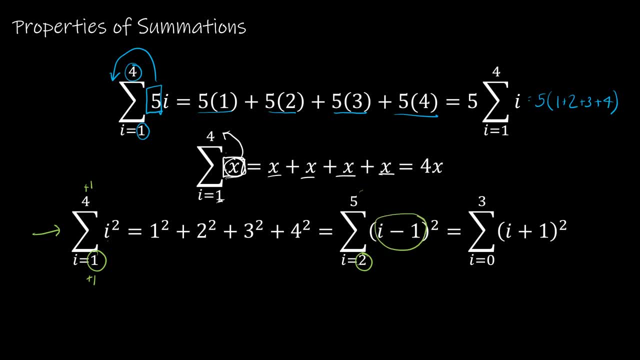 But by doing that I now have to subtract 1 from i so that it's equivalent. So 2 minus 1 is 1, so 1 squared. and then 3 minus 1 is 2, 2 squared. We get the idea It's going to be the same. 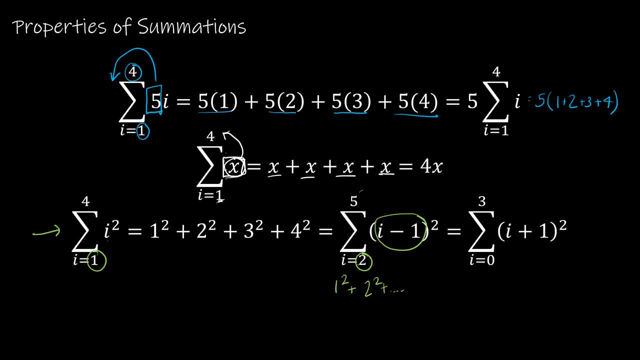 And I can also go in the opposite direction. So if I subtract 1,, then i goes from 0 to 3, and notice, then I would have to add 1 here. So 0 would be 0 plus 1, or 1 squared, and then add 1 to get 1.. 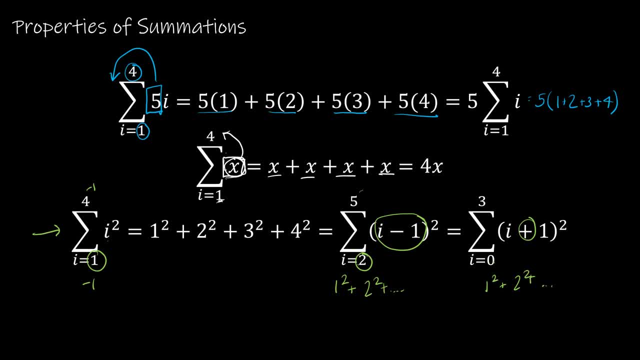 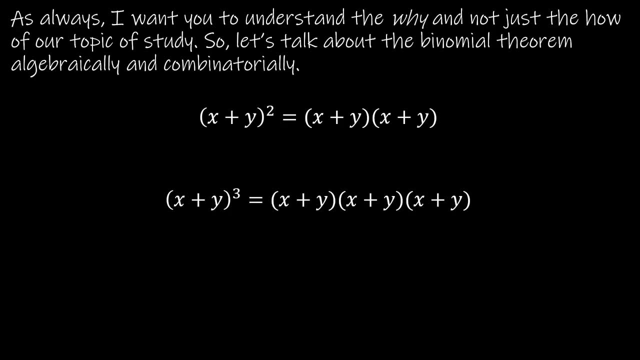 So 1 plus 1 is 2 squared, and so on. So those are just some properties that will be helpful for you moving forward. One last thing before we take a look at the binomial theorem, and that is just to develop some understanding of. 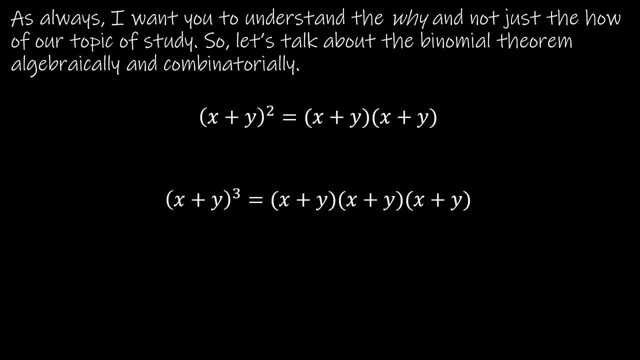 what we're actually going to be doing with the binomial theorem. So here I have x plus y quantity squared and x plus y quantity cubed. We'll start with the x plus y quantity squared, which is of course x plus y times x plus y. 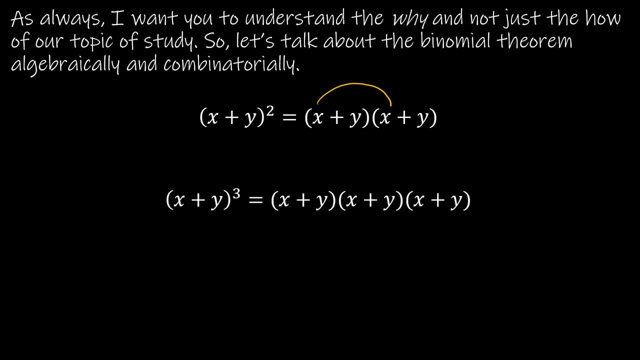 Now everybody hopefully knows how to FOIL First times. first, Outside, that's plus xy, Inside, that's plus yx, which we're going to write as plus xy, And then last, Which is plus y squared, and that's where we get Mr FOIL. 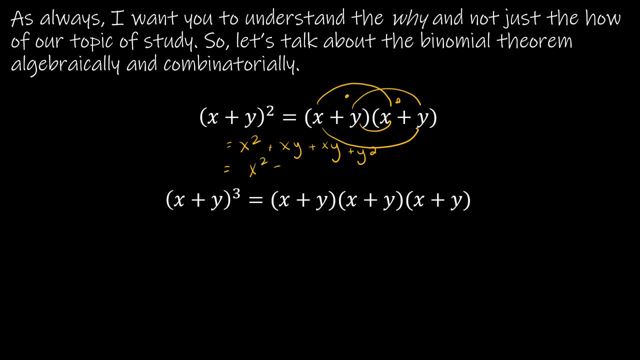 So reducing that or simplifying that a little bit, I just get x squared plus 2xy plus y squared. Now, before we look at x plus y- quantity cubed, we want to take a look at what this looks like combinatorially. 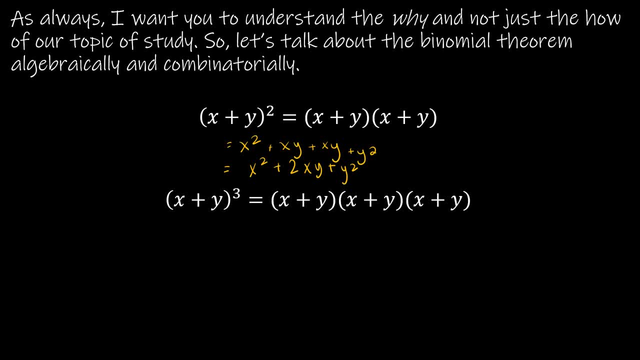 And when I say combinatorially, I mean we're looking at how we can choose the number of ways to get x squared or to get xy and so forth. So, for instance, to get x squared, there's just one way to do it. 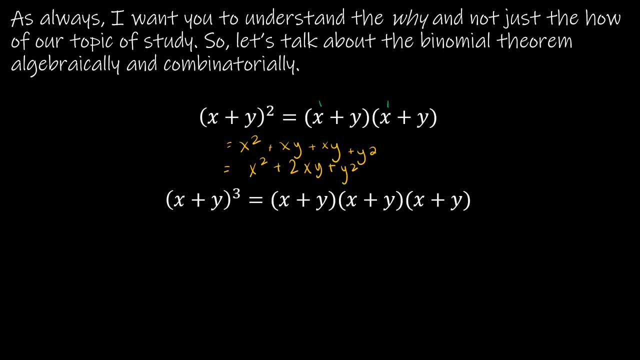 and that's to take x from each of the pairs. However, if I'm going to take xy, I could get x from the first and y from the second, or x from the second and y from the first. So that's where we're going to get that 2 combinatorially. 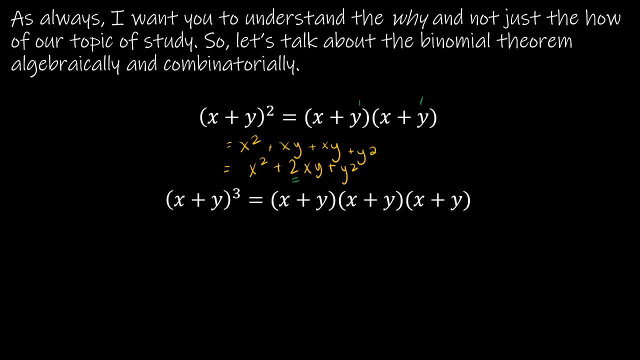 And then, of course, with y squared- it's just one way- taking y from each of the pairs. Now let's take a look at x plus y quantity cubed, which I'm just going to take this result and take it times: x plus y. 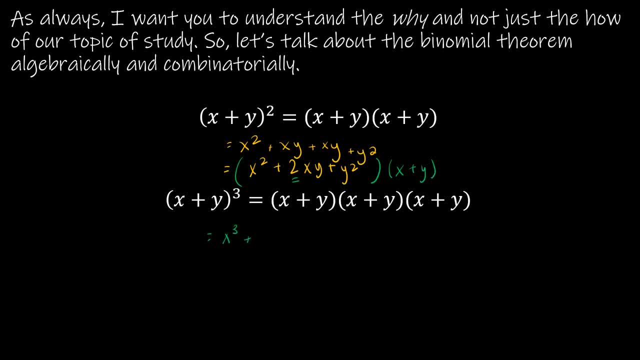 So I'm going to distribute the x, So x cubed plus 2x squared y plus xy squared, And then I'm going to distribute the y, So x squared y plus 2xy squared plus y cubed, And then I'm going to simplify. 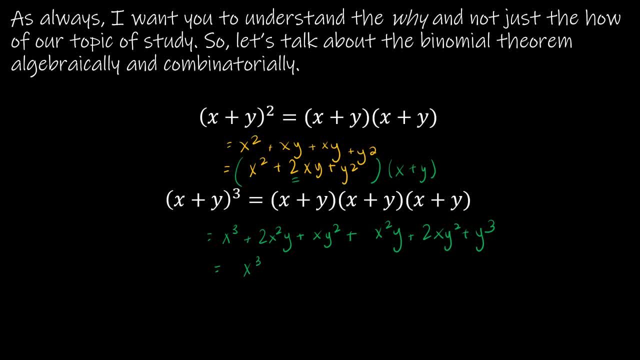 So I've got x cubed. I've got 2xy, 2x squared y and another x squared y, So that's 3x squared y. I've got xy squared and 2xy squared, So that's 3xy squared. 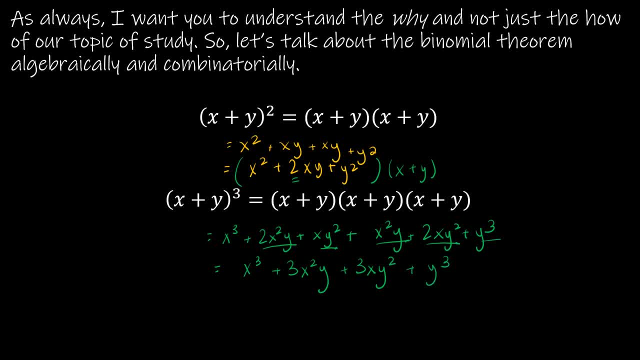 And then I've got y cubed Again, looking at that combinatorially, the only way to get x cubed is just to take x from each of the pairs. So I'm going to take x cubed, I'm going to take the x from each. 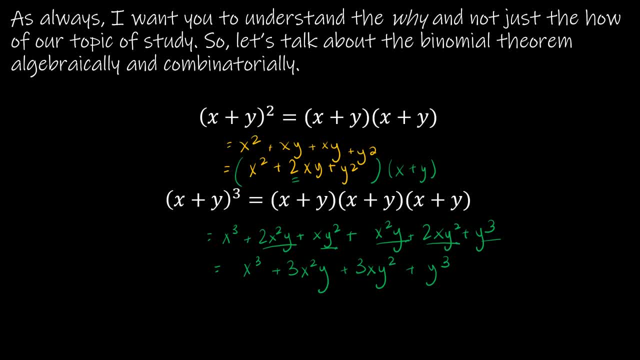 But now we've got a lot of ways that we can find x squared y, because I can take the two x's and the y. I could take an x and a y and an x, Or I can take a y and an x and an x. 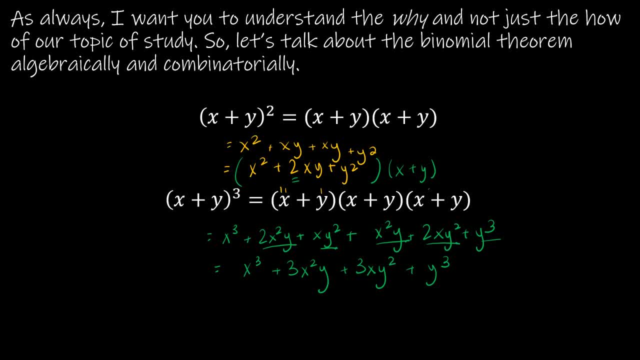 So that's where we get all three of those, And then so on and so forth. So we get the idea. So now we're going to take a look at the binomial theorem, But before we do, I just want to point out: 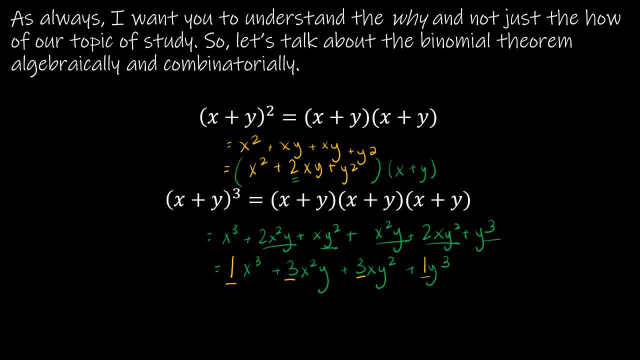 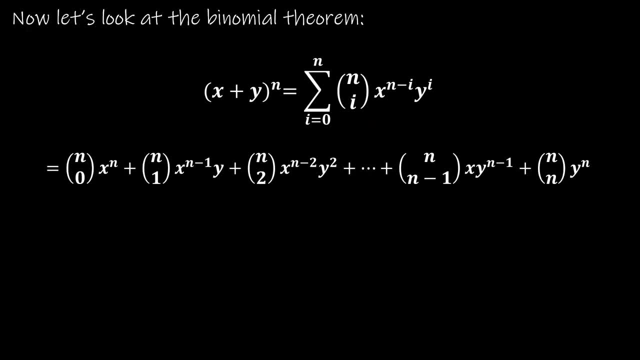 there's a 1, a 3,, a 3, and a 1.. And this one is a 1.. And this will make sense in our next video when we talk about Pascal's triangle. So, finally, we are at the binomial theorem. 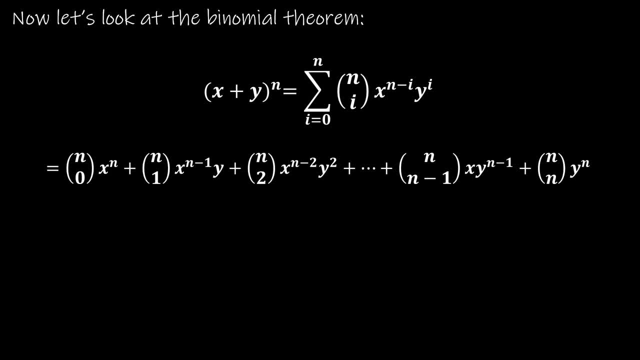 The binomial theorem says if you have x plus y to the nth power, that is the same as taking the summation. So that's why we reviewed that summation notation. The index will go from 0 to n. so whatever that last value is, 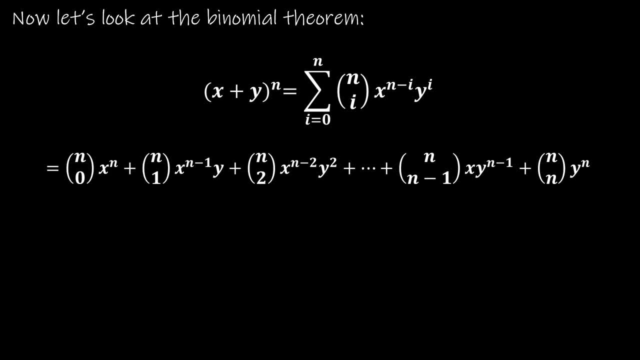 And then n choose i, And then x to the n minus i, y to the i. So this is just another representation of that, obviously symbolically, But let's go ahead and take a look at x plus y squared that we just found together. 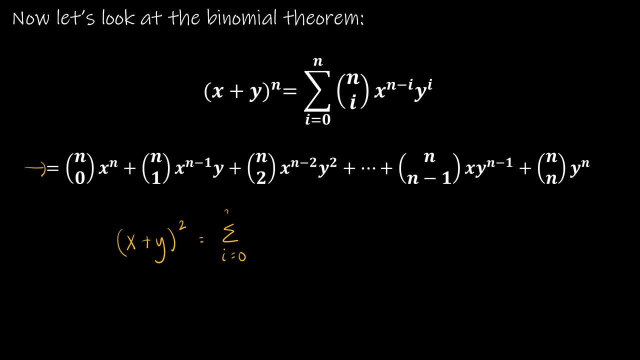 That tells me I'm going from 0 to 2 of n. choose i. So n again was b2.. Choose i. And then we had x to the n minus i, y to the i. So what does that tell me to do? 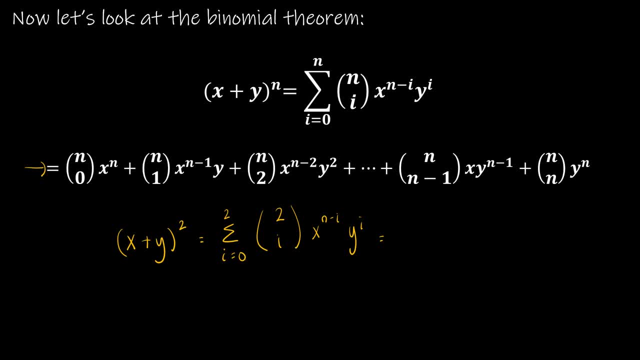 That says start at 0.. The first term is 2, choose 0. And then it would be x, So I'm right here, x to the 2 minus i, so 2 minus 0. And then y, And then y to the i, and again i is 0. 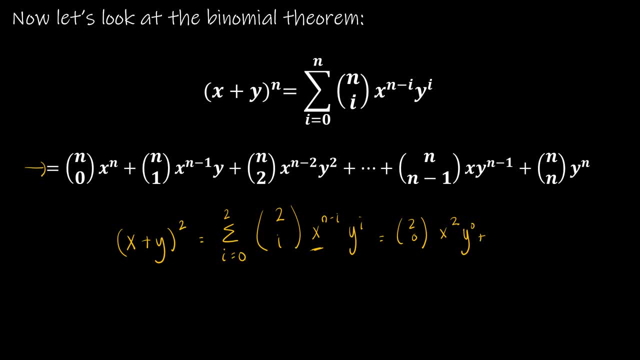 So y to the 0.. And then we move on to: i is equal to 1.. So if i is equal to 1, it's 2, choose 1.. And then x to the 2 minus 1, which is 1.. 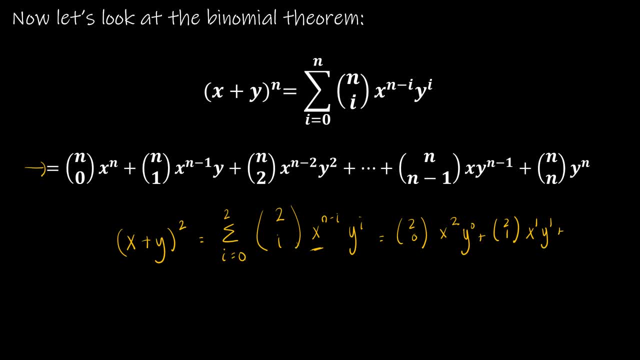 And y to the i, which is 1.. And then move on to 2.. So 2 choose 2.. And then x to the 2 minus 1.. And then x to the 2 minus 1.. And then y to the 2 minus 2.. 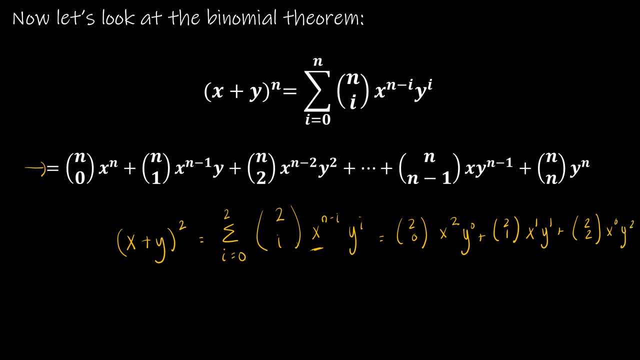 So x to the 0.. y to the 2.. So what does that tell me? Well, 2 choose 0.. There's only one way to choose, And that gives me x squared And then y to the 0.. 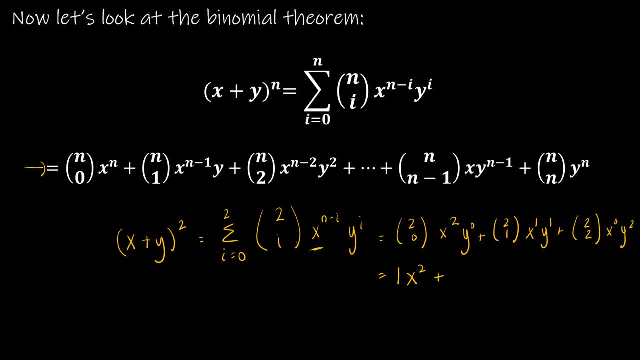 So we're not going to write that. And then 2 choose 1 is 2.. Remember we just talked about this. This is 2 factorial over 1 factorial, 1 factorial, 2 minus 1 factorial, Which is 1 factorial. 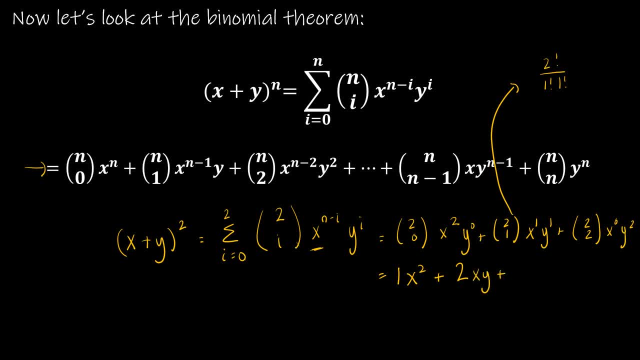 So that gives me 2.. And then x to the first, y to the first, And then 2, choose 2.. Again, 2 factorial over 2 factorial, 0 factorial. That's going to give me 1.. x to the 0, again is 1.. 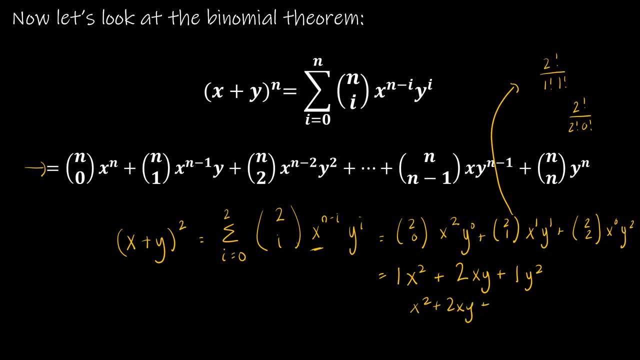 And then y squared. So really, I just got x squared plus 2xy plus y squared, Which, if you'll recall, was what we got when we foiled this out. I can do the same thing for cubed and get the same result. 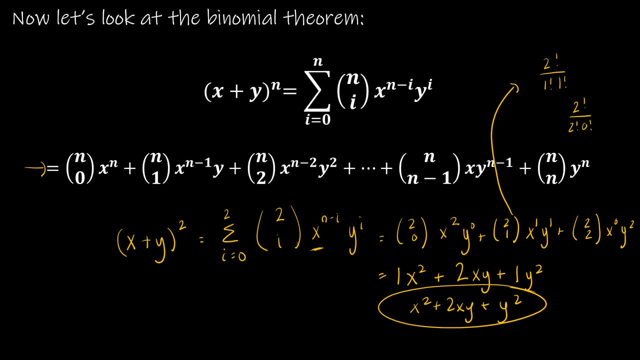 I don't, I'm not going to do that just for the sake of time in this video, But that's all this mumbo jumbo is telling you Is essentially: this value is going to keep increasing. So 2, n choose 0,, n choose 1, n choose 2, and so on. 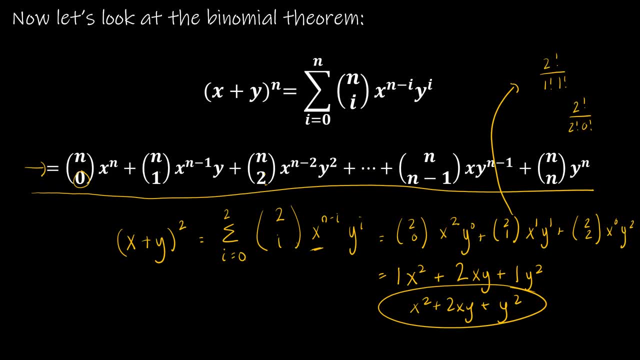 Until you've made it to the end of the list And your exponent on your x value is going to start at n and continue to decrease By 1.. Your y value is going to start at 0. And continually increase by 1 until you reach n. 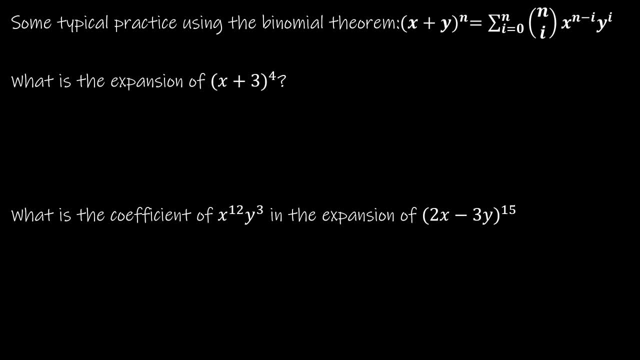 Let's look at two traditional practice or typical practice using the binomial theorem, And these are just direct application of the binomial theorem. So the first one asks us to just find an expansion. So again, we're just going to be using the summation. 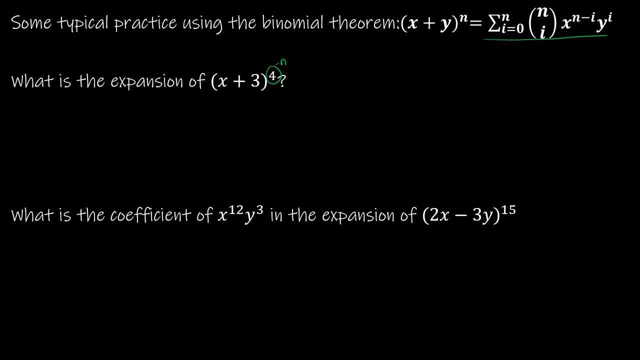 So n obviously is 4.. And we're starting at i is 0.. So we're saying 4, choose 0.. And then the first term to the fourth power, And the second term, which is different this time, is not a y. 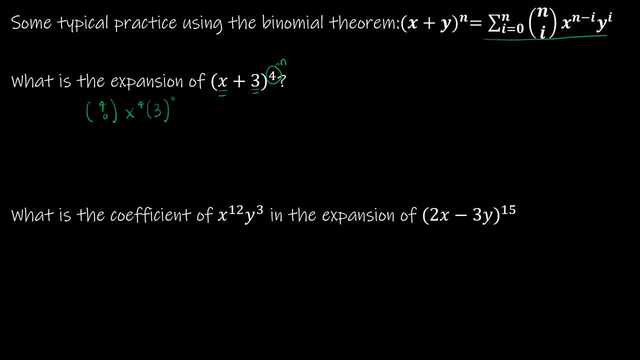 But is an actual constant And that's going to be to the 0 power. So I'm just going to write it all out, initially And again: the x value, the exponent, is going to decrease by 1.. The y is going to decrease. 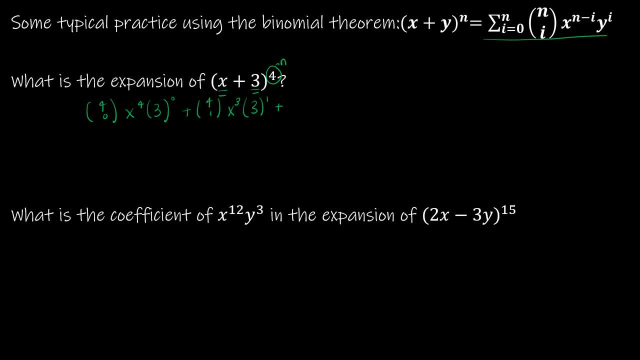 The y value, which in this case is 3.. The exponent is going to increase by 1. And then we'll do some simplification, So that's supposed to be a 2.. 4 choose 2.. x squared, 3 squared. 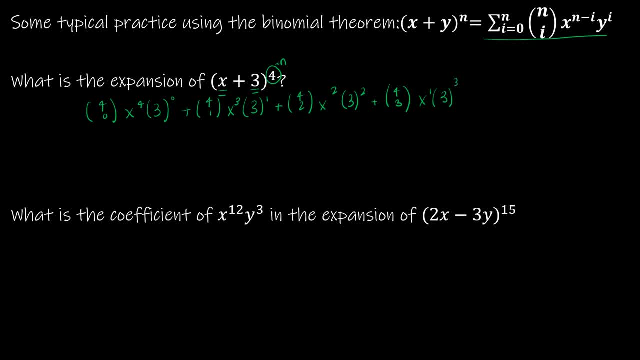 And then 4, choose 3.. Decrease x by 1.. Increase 3 by 1.. And then 4, choose 4.. And then x to the 0.. 3 to the fourth- All right, So now let's take a look at how we can reduce this. 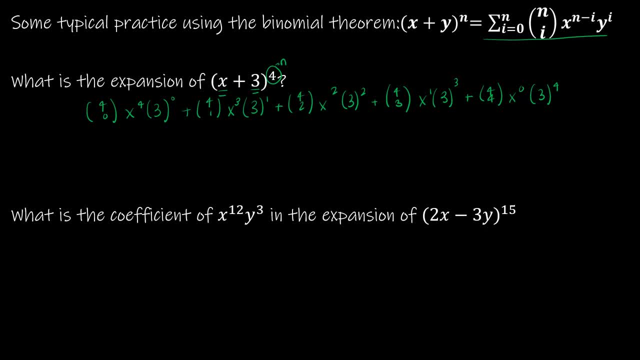 So obviously, yes, I wrote the expansion, But this would not be an acceptable solution because I haven't reduced anything or made it pretty, I guess. So 4 choose 0 is 1.. But if you'll notice, here I also have to take into account that I've got another number, not variable. 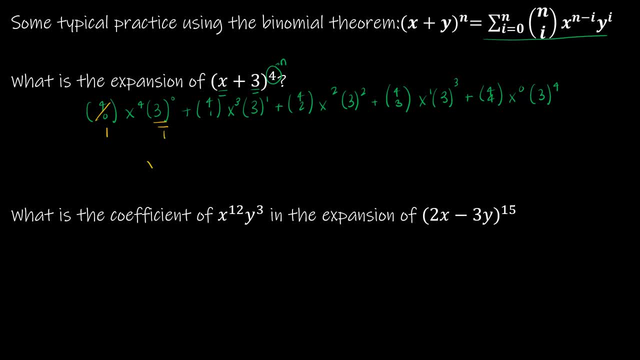 So 3 to the 0 is 1.. So that gives me 1 times x to the fourth. So x to the fourth is my first term. 4 choose 1 is 4.. But again, I've got 4 and I've got 3 choose 1, which is 3.. 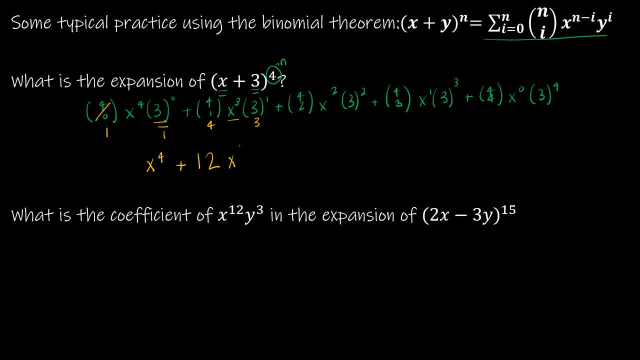 So this is actually 12 x to the third, And then 4 choose 2.. Remember, all we're doing to find those solutions is 4 factorial, 2 factorial. 4 minus 2 factorial, That's going to give me 6.. 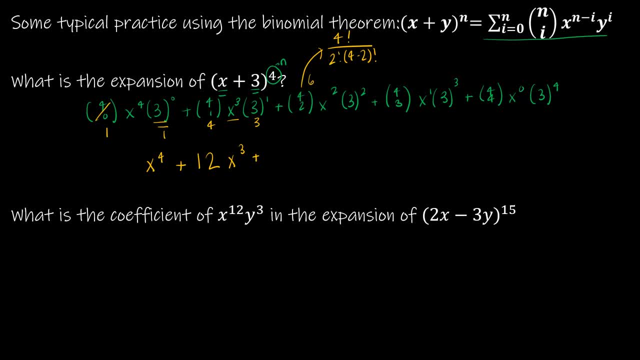 So if you don't recall that, make sure you go back to the combinations video. This would be 6.. But then this guy is 9.. So 6 times 9 is 54 x. squared Again, 4 choose. 3 is going to end up as 4.. 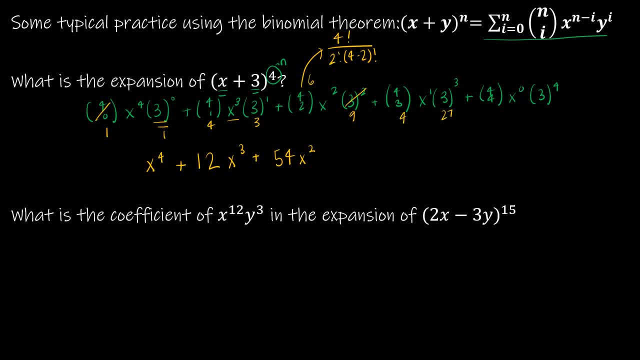 And then 3 to the third is 27.. So we're going to multiply that out to get 108.. x And then 4: choose 4 is 1. And 3 to the fourth is 81. So that gives me plus 81.. 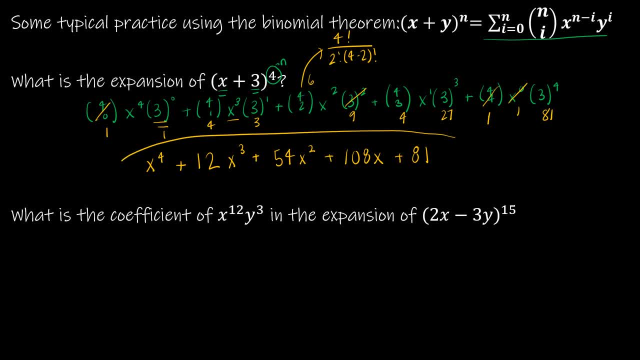 And x to the 0,, as we know, is just 1.. So that is the expansion, And again, that might not seem like a fast way to find the solution, But it's a lot faster than having to FOIL everything out. 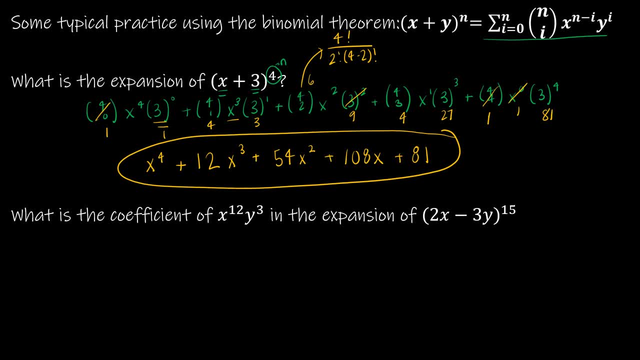 And then distribute, and then distribute some more in combined like terms. The other type of question that I'm going to ask you is- and this is one that you'll get most often- is one where they ask you just to find the coefficient. So, again, it's going to be the same idea as what we just did. 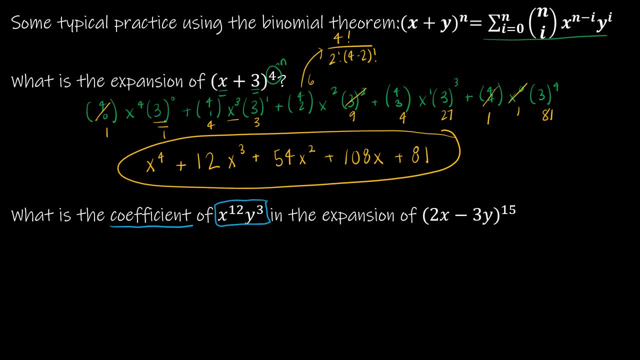 but we're only going to focus on the coefficient for one value. The biggest mistake that I see students make here is again forgetting that if you've got numbers, like we did here, you have to take those numbers into account when finding the coefficient. 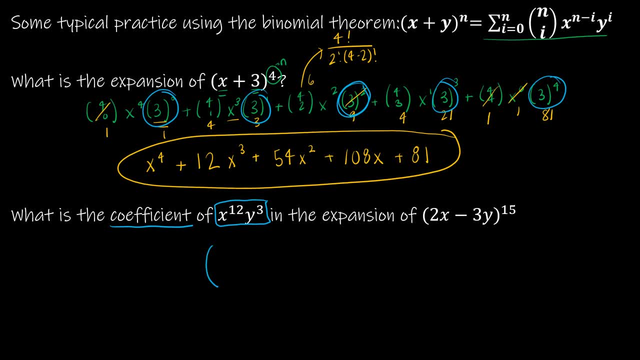 So what I'm going to do here is essentially: you're going to take the 12 plus 3 to find that n is 15.. So it's 15.. Those will always add up to n. So 15, choose, and it's going to be whatever the second value is. 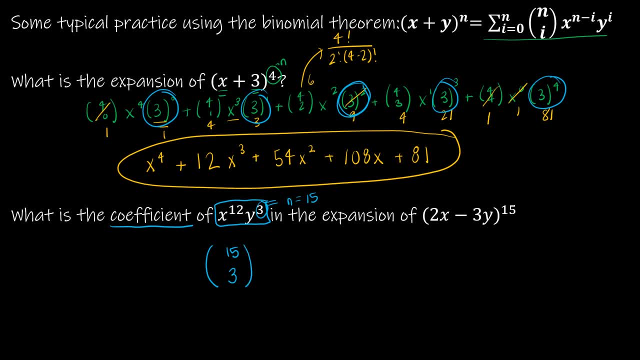 So 15 choose. 3 is the first part of our solution, And then the first value, in this case 2.. So it's 2x. But again, I'm only looking for the coefficient, so I don't care about the x. 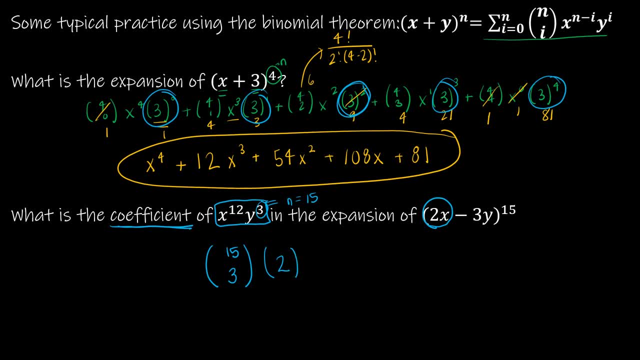 I only care about the 2.. I'm going to take 2 to the 12th power and I'm going to take negative 3.. Again, I could put the y in there, but I don't care. Negative 3 to the third power. 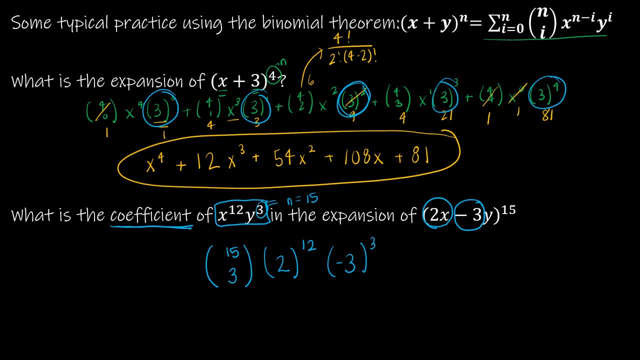 And then I'm just going to use my calculator So you can find each part separately for 15,, 455,, 4096, negative 27, and then multiply those out, Or you can just get your calculator out and do it all. 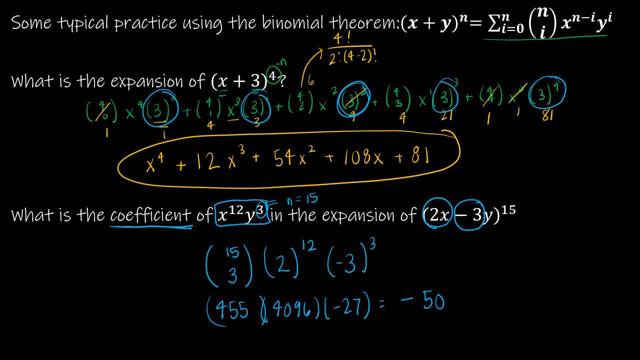 And either way you're going to end up with- let me write it down before I say it so I don't screw it up- negative 50,319,360.. So again, very large number, but made very easy by using the binomial theorem. 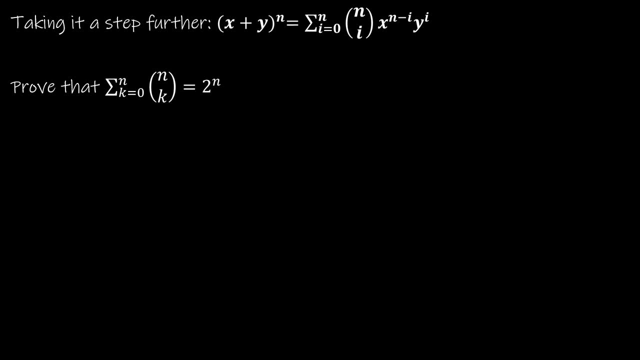 I do want to take it just a step further and do a quick informal proof, so I'm not going to write out all of the steps. I'm just going to give you an idea of how we can use the binomial theorem in a proof like this. 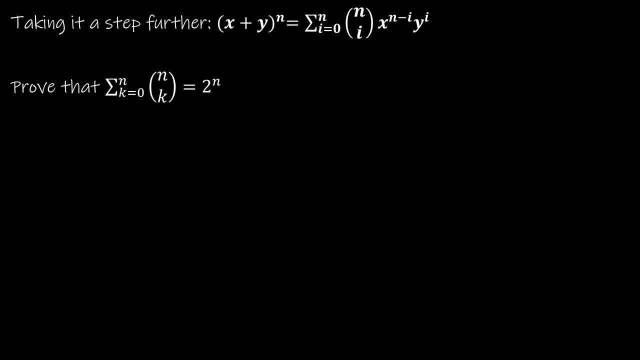 So what we're asked to prove is that the summation, as k goes from 0 to n, of n- choose k- is equal to 2n. So if you'll notice, this part of our expression closely matches this part of our expression. 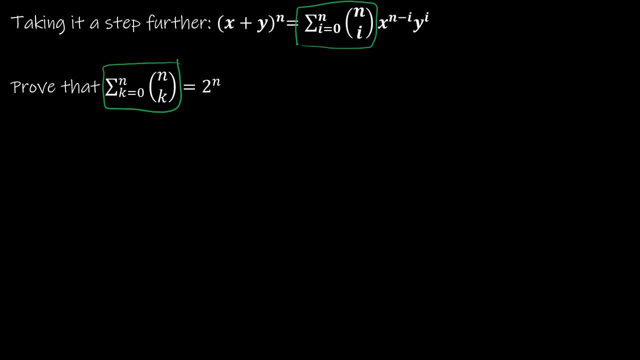 So how is that helpful to me? Well, because I can say that 1 plus 1 to the nth power is the summation as i goes from 0 to n of n choose i, and then 1, to the n minus i. 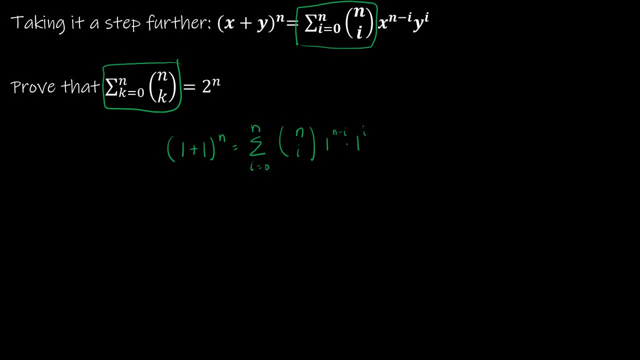 times 1 to the i. Well, 1 to any power is 1, and 1 to any power is 1, so really these don't matter, But what we're saying is 1 plus 1, which is 2,. 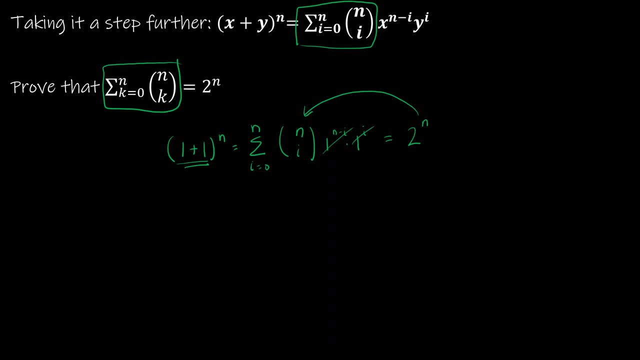 2 to the n is equal to the summation. as i goes from 0 to n of n, choose i. Well, does that look a heck of a lot like this? Yes, So instead of using i, they're using k.